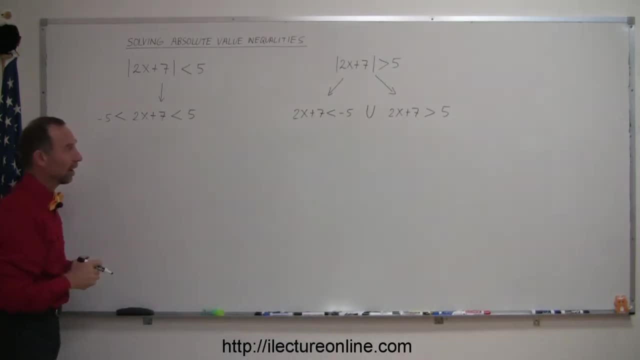 so you use the union symbol, meaning both conditions must be satisfied. All right, so that's how you deal with these. Now let me show you how to complete the problem. Well, the first thing you want to do here is: you want to isolate x. that means you want to get rid of everything else. You want to get rid. 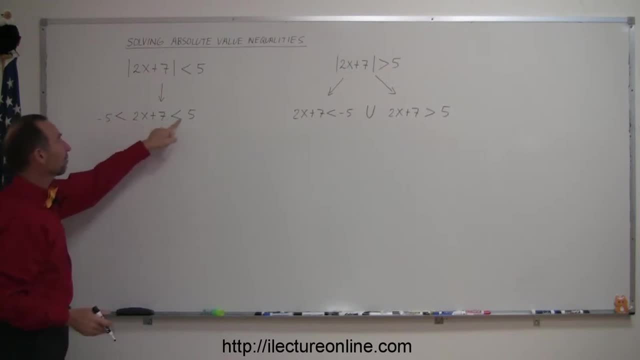 of the 7. that means you want to subtract 7 from the left, from the middle and from the right side of the problem, and let me use a different color to illustrate that. So you want to get rid of everything else. So you want to rewrite this as: minus 5, less than 2x, plus 7, less than 5, and, of course, 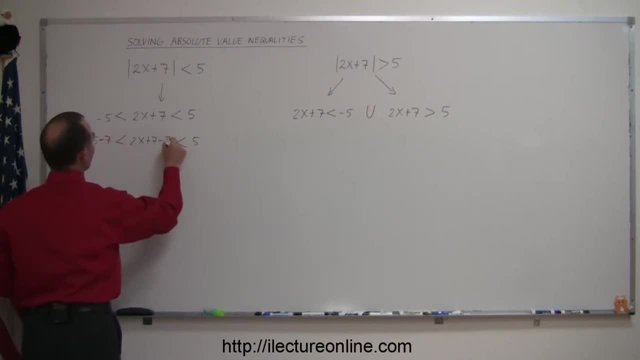 you want to subtract a 7 from there, from there and from there. that means everything is still the same. but notice, when you do that here, the 7s disappear and minus 5 minus 7 is minus 12, less than 2x, which is less than 5 minus 7, which is minus 2.. Next thing you want to do is get rid of the 2, so you're. 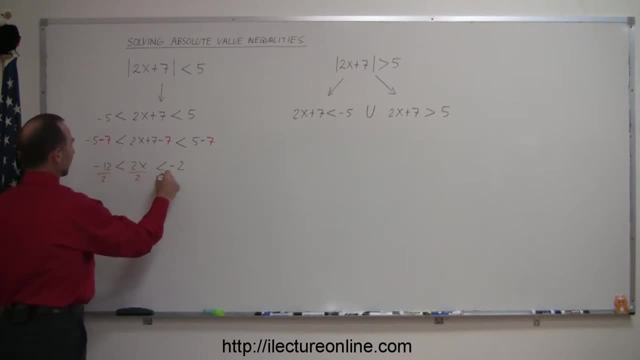 going to divide that by 2. so let me illustrate that in red: divide that by 2, divide that by 2, divide that by 2 and now we get minus 12. divided by 2 is minus 6, less than x, which is less than. 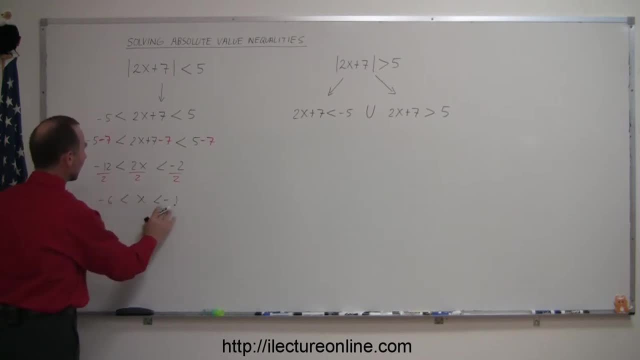 negative 1.. So here it tells you that x must lie between negative 6 and negative 1, which could be illustrated graphically: if this is 0 and this is negative 1 and this is negative 6.. Notice that negative 6 and negative 1 are not included, because it doesn't say less than or equal to, and everything. 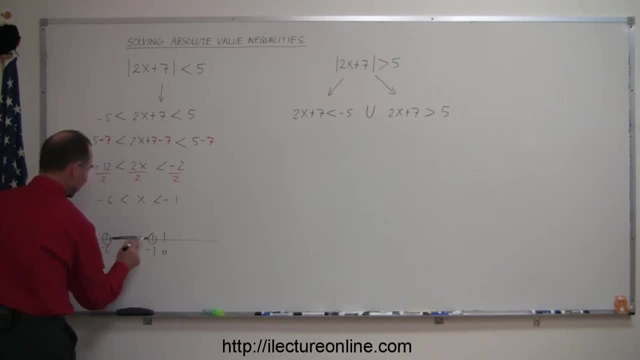 is between. so we can darken that up with a solid line, and so this graphically illustrates: we're looking for all values between negative 1 and negative 6.. So this is how you do that when you have a case like that Now over here, you have to work those separately. you want to solve for x, so 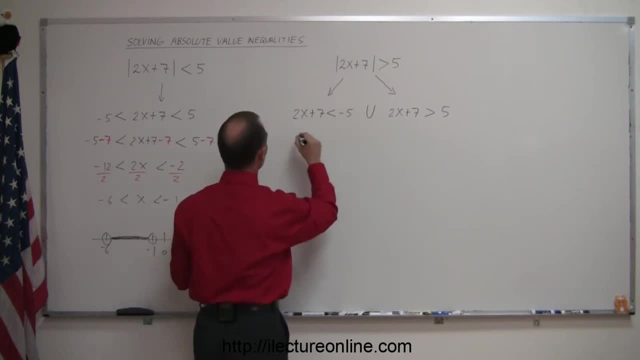 you're going to, in this case you're going to subtract 7 from both sides. so let me write that 2x plus 7 less than minus 5. so I'm going to subtract negative 7 from both sides. negative 7, negative 7 like so. 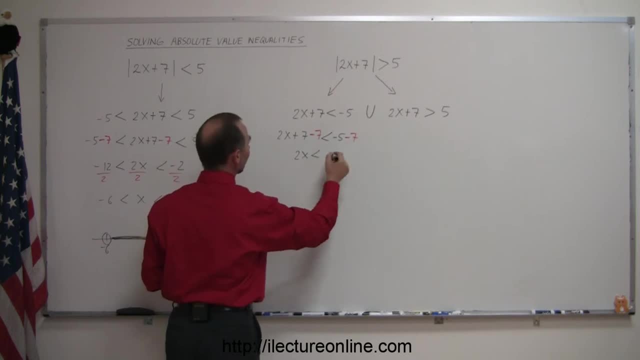 Then we get 2x is less than minus 5, minus 7 is minus 12, and then you divide both sides by 2 and you can see that on the left side here you get x is less than negative 6, and at the same